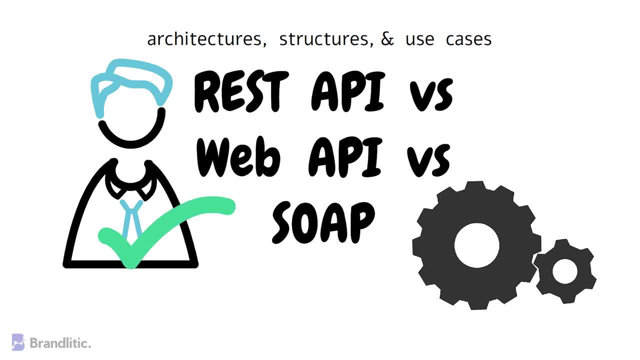 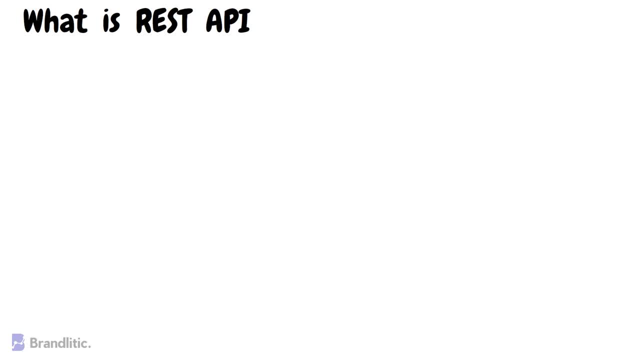 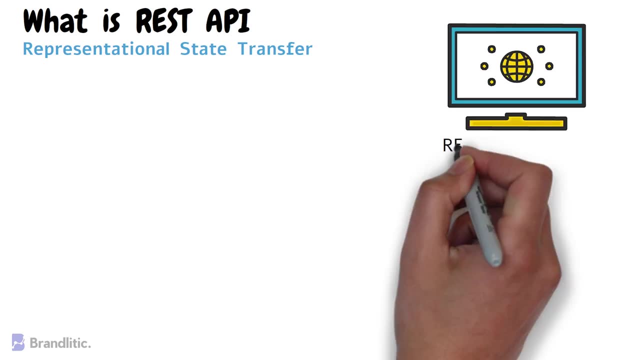 between each one of them and when to use each one of them. So let's get started. First off, what is REST API? Well, REST stands for Representational State Transfer, and REST API is a web-based application programming interface that follows the REST architectural style. The primary purpose of REST is to provide 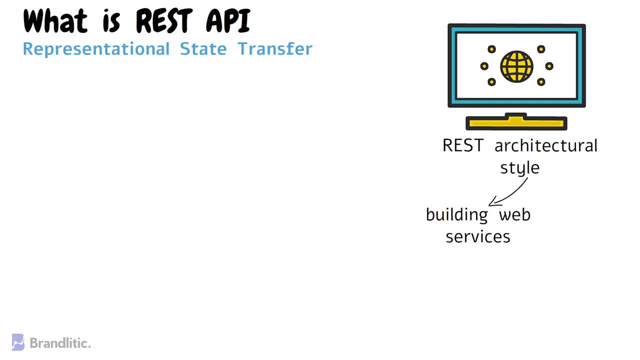 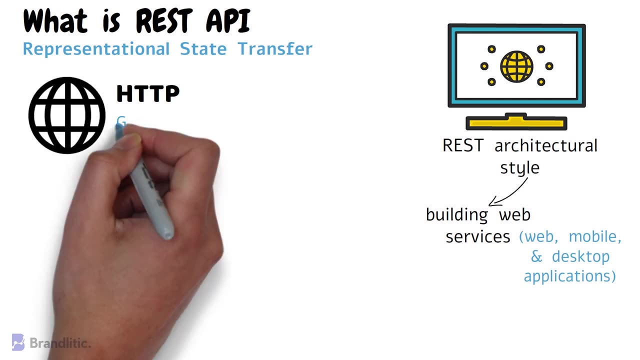 an architecture for building web services that can be consumed by various clients, including web, mobile and desktop applications. REST is based on HTTP, which is the standard protocol used for communication on the internet. It uses the HTTP method, including GET, POST, PUT, DELETE, etc. to perform various operations on the resources. Each resource in REST is: 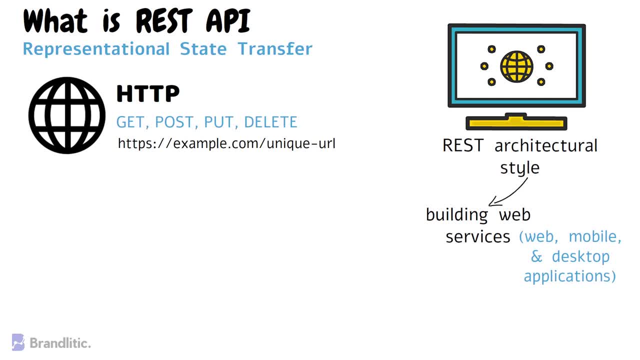 identified by a unique URL and the response is returned in JSON or XML format. One essential feature of REST API is that it follows the stateless client-server model. This means that the server doesn't store any information about the client's internet service. Instead, each request contains all necessary information required by the server. 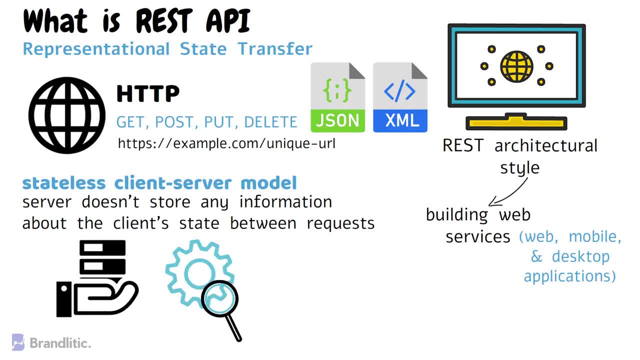 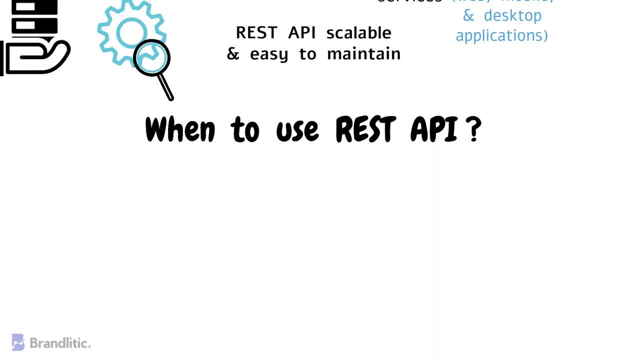 to process the request. This architecture makes REST API scalable and easy to maintain. So when to use REST API? Frankly speaking, REST API is an excellent choice when building web services that require stateless, scalable and easy-to-maintain architecture. It's ideal for building applications that require CRUD operations, such as CRUD. 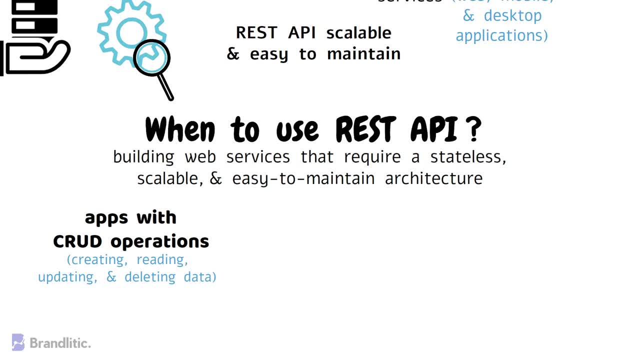 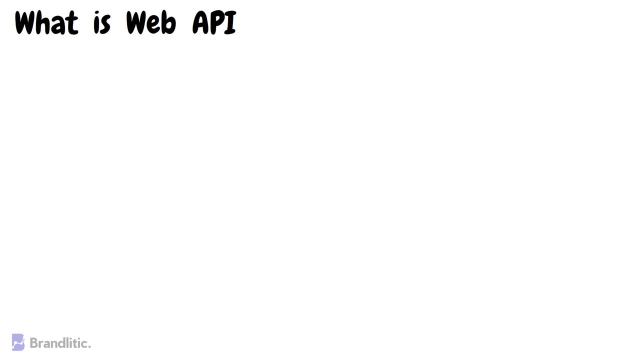 such as creating, reading, updating and deleting data. REST API is also suitable for building applications that require real-time communication, such as chat applications and streaming services. What is Web API? Well, to state simply, Web API is a broader term that encompasses all. 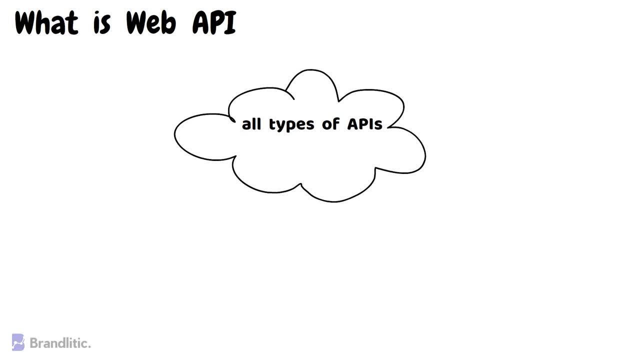 types of APIs that can be accessed over the internet. It includes REST API, SOAP, XML, RPC and many others other types of APIs. The primary purpose of Web API is to provide a platform-independent interface that can be used by various clients, including web, mobile and desktop applications. 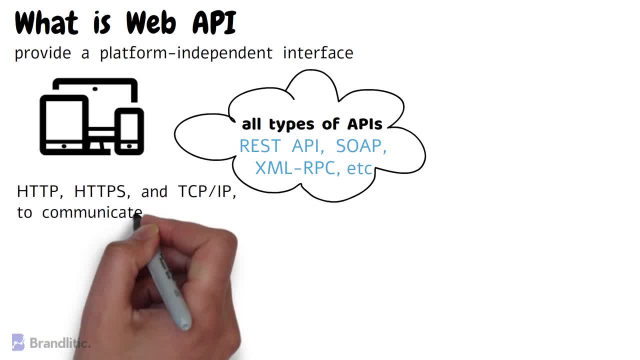 Web API uses different protocols, including HTTP, HTTPS and TCPIP, to communicate between clients and servers. Unlike REST API, Web API doesn't follow a specific architecture or structure. Instead, it can be designed using any technology or architecture, depending on the requirements. 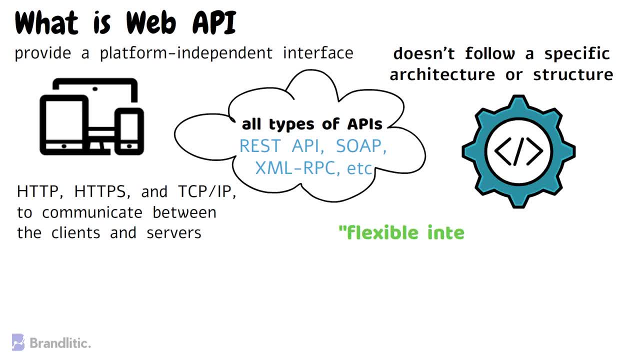 One of the key features of Web API is that it provides a flexible interface that can be used by various clients, and it allows developers to expose various functionalities of the application, including thread operations, authentication, authorization and many others. This makes Web API a powerful tool for building complex applications that require a lot of 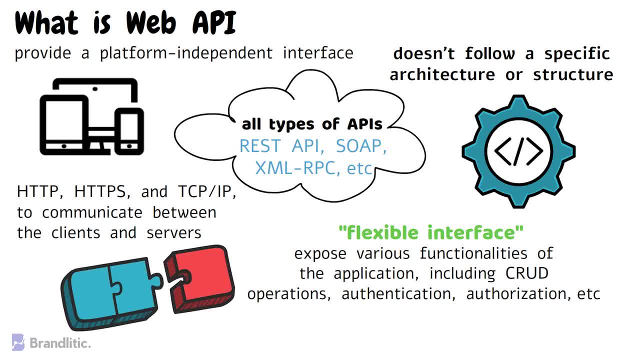 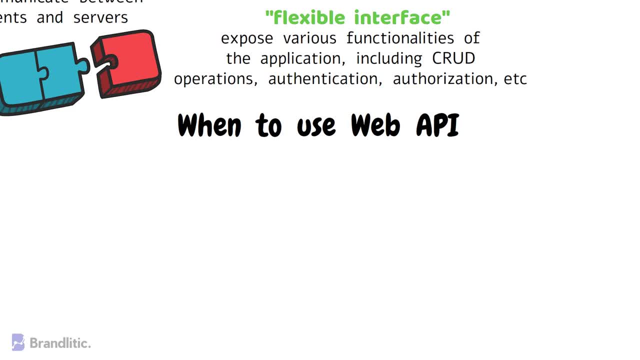 integration and communication between different systems. So when to use a Web API? Frankly speaking, Web API is a better choice when building complex applications that require integration with different systems and technologies. Web API provides a flexible interface that can be customized to meet the requirements. 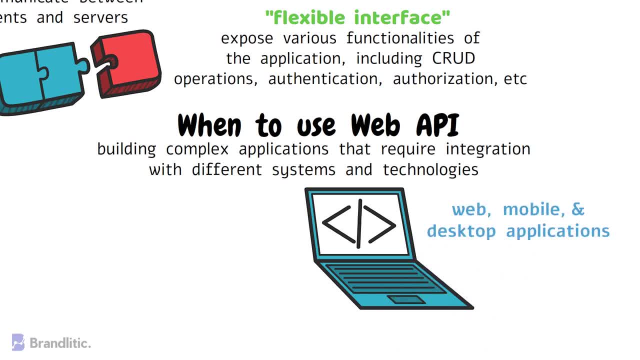 of various clients, including web, mobile and desktop applications. Web API is also suitable for building applications that require authentication, authorization and security. Next up Web API is a great tool for building complex applications that require authentication, authorization and security. 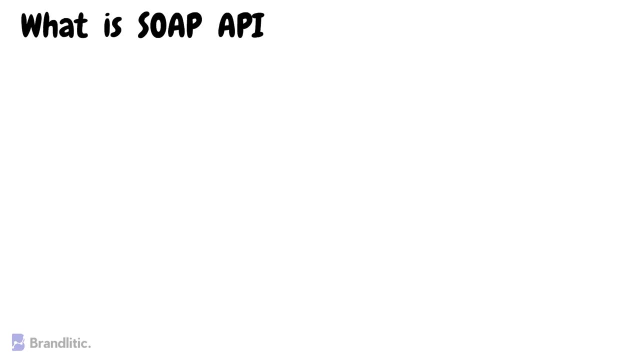 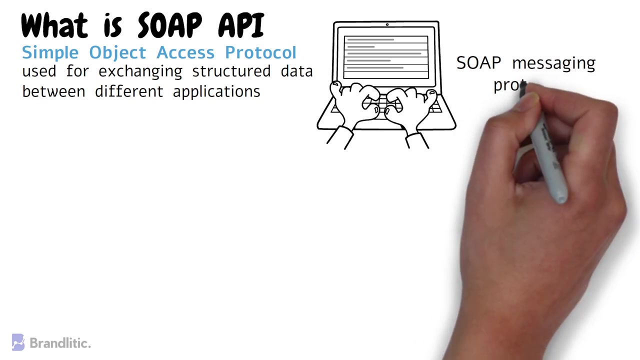 Next up. what is SOAP API? Well, SOAP stands for Simple Object Access Protocol, which is a messaging protocol used for exchanging structured data between different applications. SOAP API is a web-based application programming interface that follows the SOAP messaging protocol. The primary purpose of SOAP is to provide a standardized way to exchange data between. 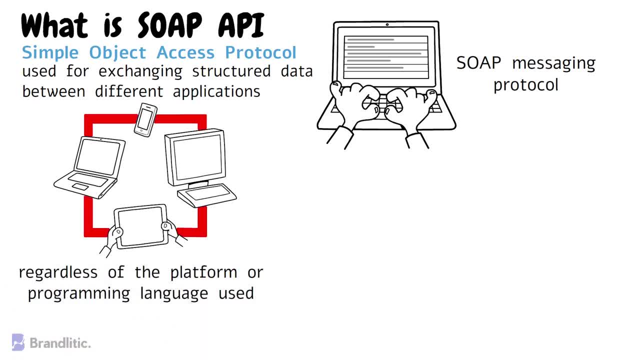 applications, regardless of the platform or programming language used. SOAP API uses XML as the format for SOAP. It provides a wide range of data types, including text, numbers, dates and binary data. SOAP also supports multiple transport protocols, including HTTP, SMTP and FTP. 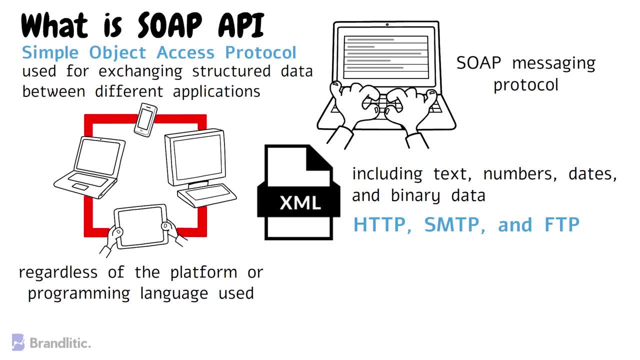 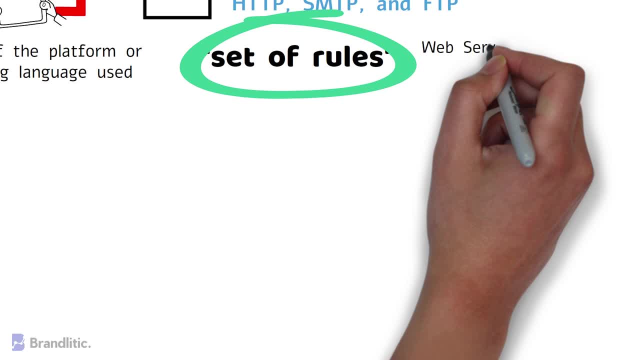 One of the essential features of SOAP API is its ability to define a set of rules for exchanging messages between applications. These rules are defined in the Web Services Description Language, or WPAP. So when to use a Web API, Well, the first step is to define a set of rules for exchanging messages between applications. 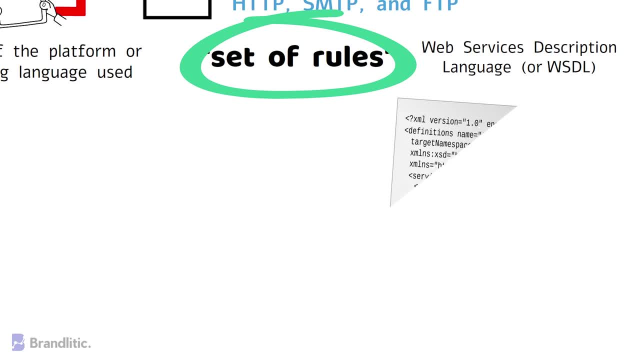 Once you have defined the conditions for your Web service, store your taxes or look for data, etc. Or you can use SSN to touching up the content. Then move the Web API to the selvesviable IP fork with functions like request automatically. 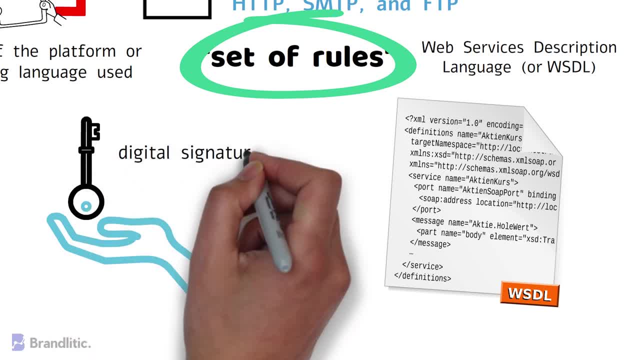 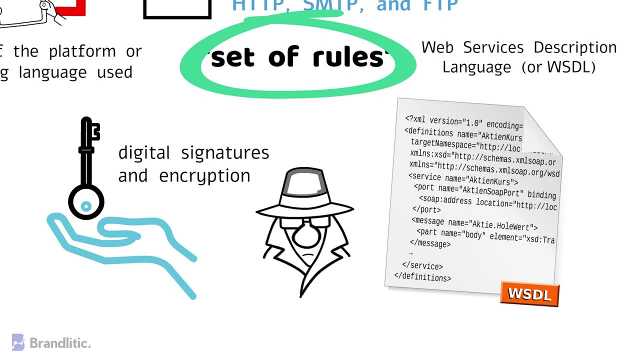 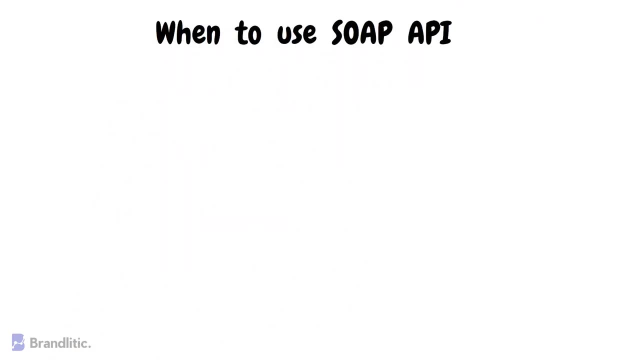 finnish androgenous. You can, of courseắnglish the webIDE service, Or uh get theை Polizei. and the SOAP API is an excellent choice when we are building applications that require a highly secure and reliable method for exchanging data between the applications. 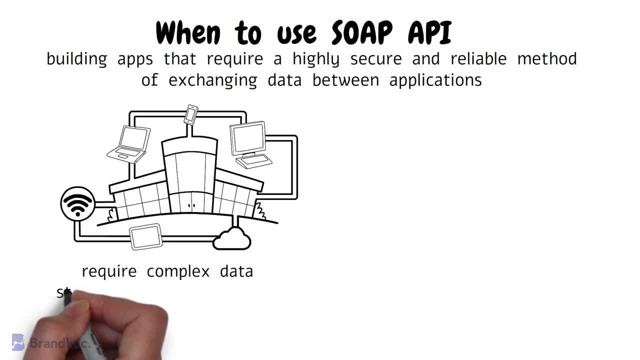 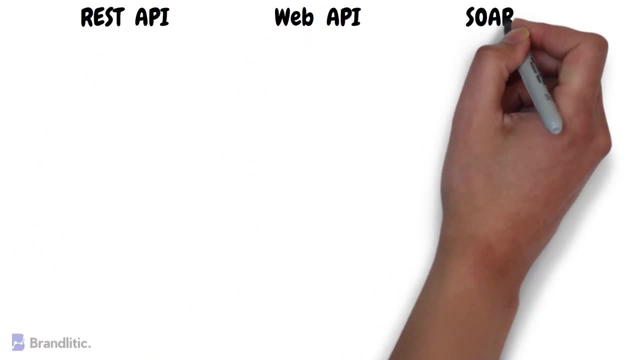 It is ideal for enterprise-level applications that require complex data structures and business logic. SOAP API is also suitable for building applications that require advanced security features, such as digital signatures and encryption. Next, let's summarize the difference between REST API vs Web API, vs SOAP API. 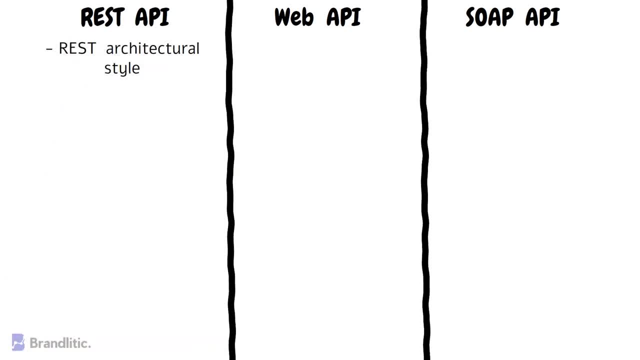 First, REST API. It follows the REST architectural style. It uses HTTP methods like GET, POST, PUT, DELETE to perform operations on resources. It returns data in JSON or XML format only and follows the stateless client-server model. It is suitable for simple applications, particularly those that require CRUD operations and real-time. 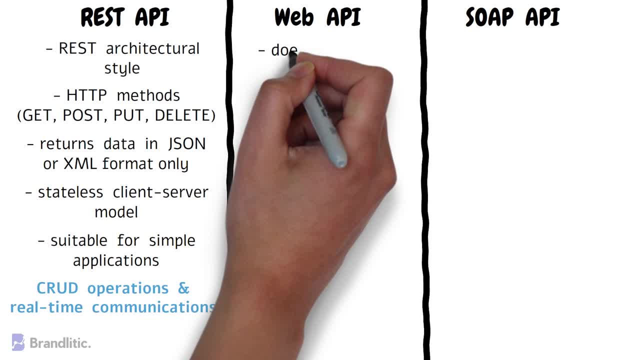 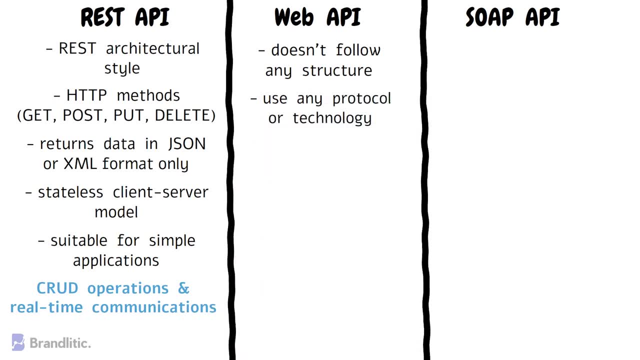 communication Next Web API. It doesn't follow any specific architecture or structure. It can use any protocol or technology to communicate between client and servers. It can use any data format, including JSON, XML, CSV and many others and further can be stateless or stateful depending on the requirements. 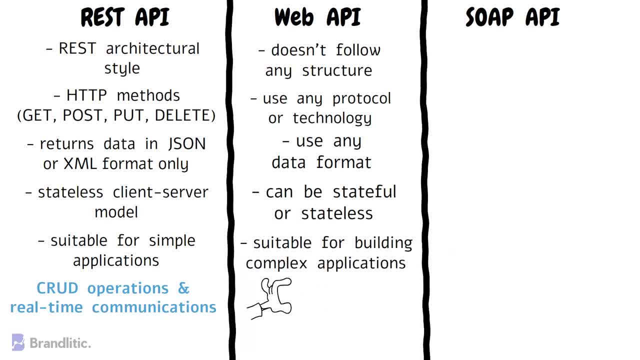 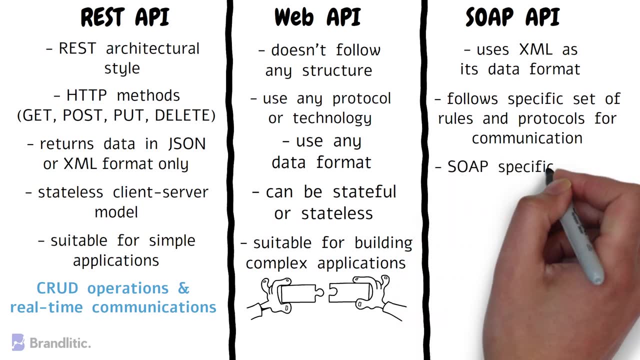 It is suitable for building complex applications that require integration with different systems and technologies. And lastly, SOAP API. It uses XML as its data format. It follows a specific system. It has a specific set of rules and protocols for communication. It requires a SOAP-specific protocol, such as WSDL or UDDI, to describe the interface. 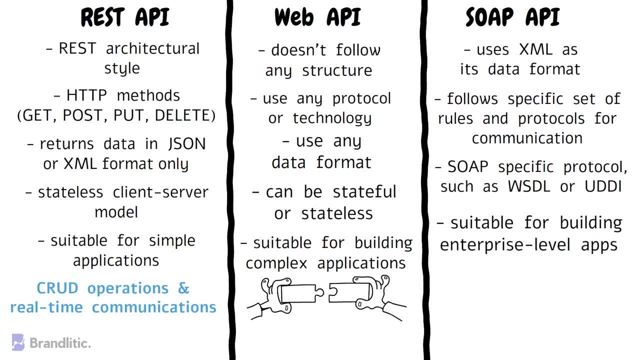 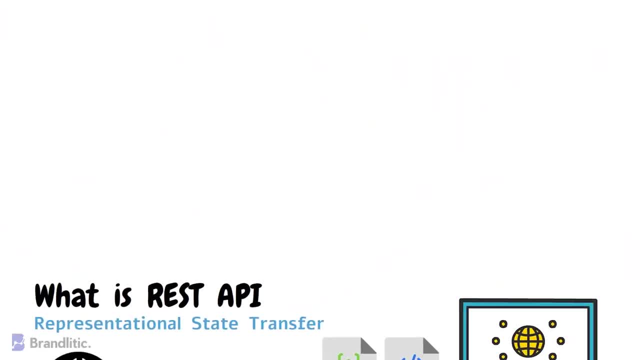 It is suitable for building enterprise-level applications that require robust security and reliability. With that, I hope this video was helpful to you and served value. If you like my content, feel free to smash that like button, and if you haven't already subscribed to my channel, please do, as it keeps me motivated. 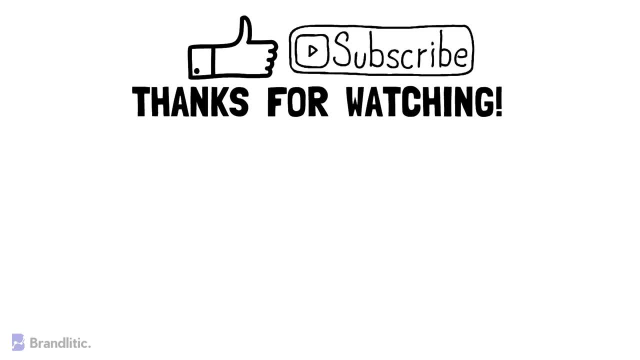 I will see you in the next video. Bye for now.